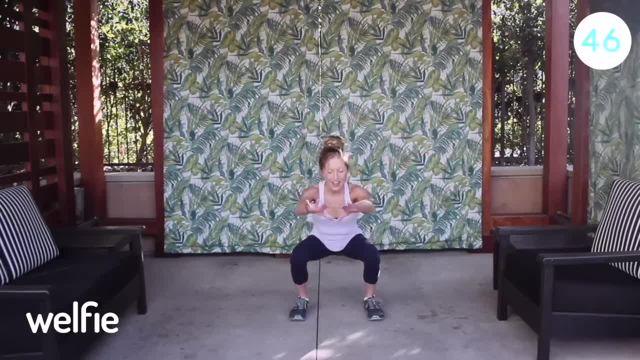 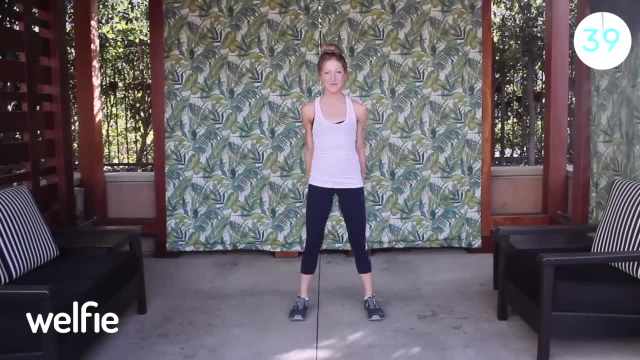 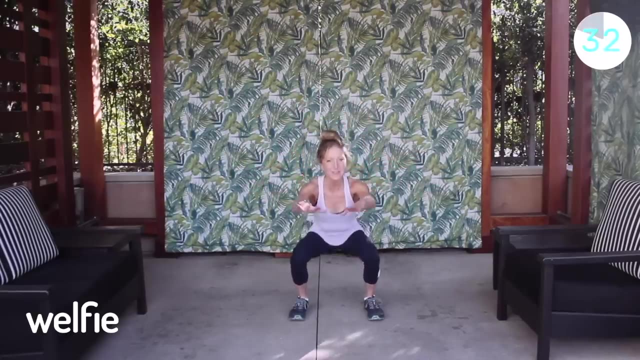 we go, Come up and squeeze your glutes. The squat can be done in a variety of ways and I've shown you many ways on how to squat on this YouTube channel. So if you haven't checked out my other diabetes exercises videos, do that so you can learn how to squat in a way that feels right for you. 50 seconds is. 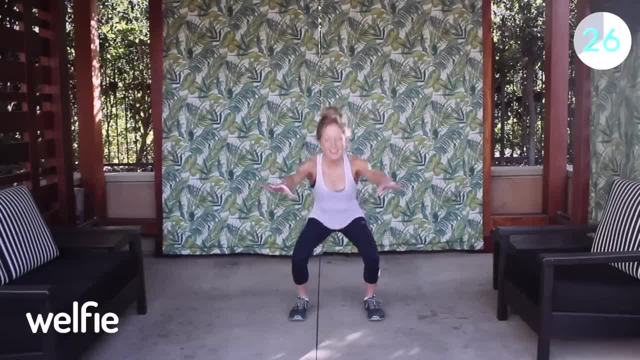 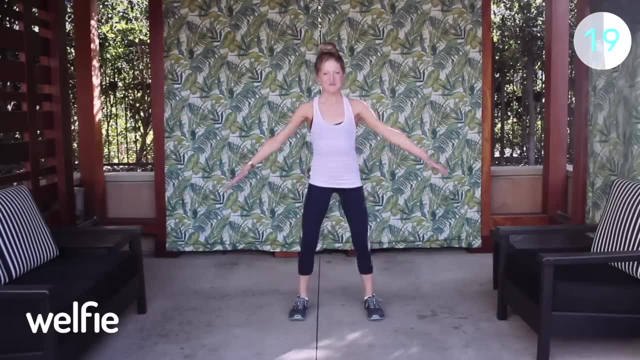 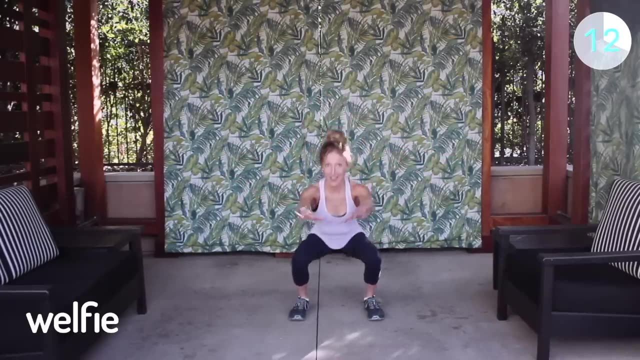 a long time when you're moving well. So make sure you breathe, think positive and keep going at a pace that challenges you. I love a good squat, Shoulders down and back chest up. Are you breathing? I hope so. That's important Stay. 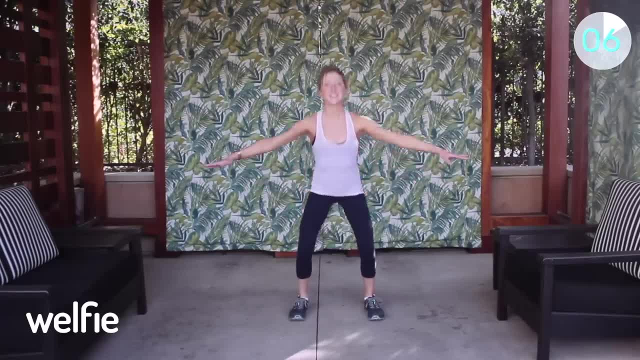 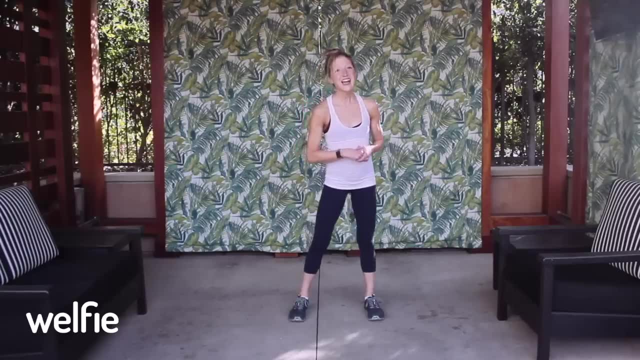 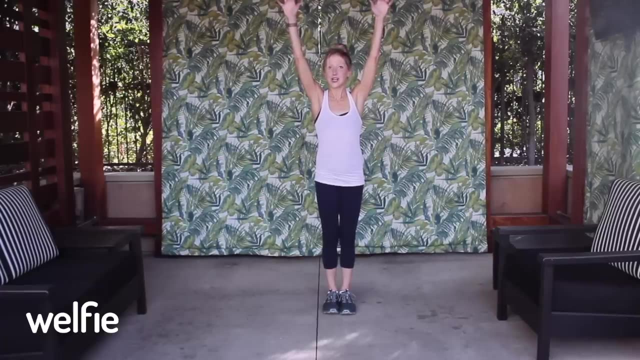 with it. Great squat to start you off for success. I bet you already feel better. I know I do. Next exercise is a knee raise 50 seconds, Arms up, tummy tight and bring your knee into your chest Go. 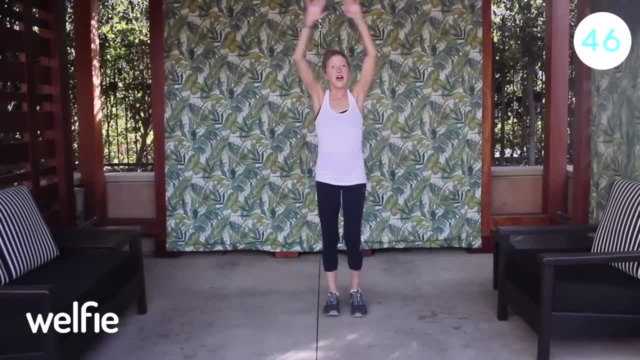 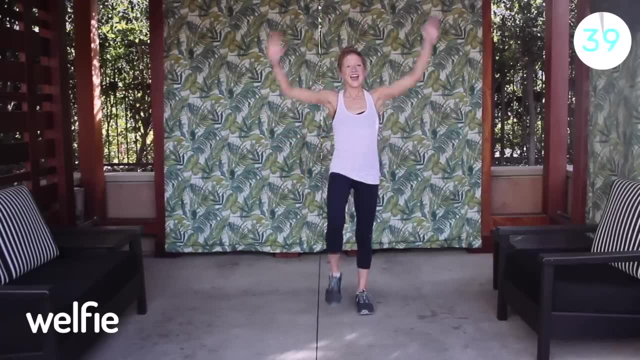 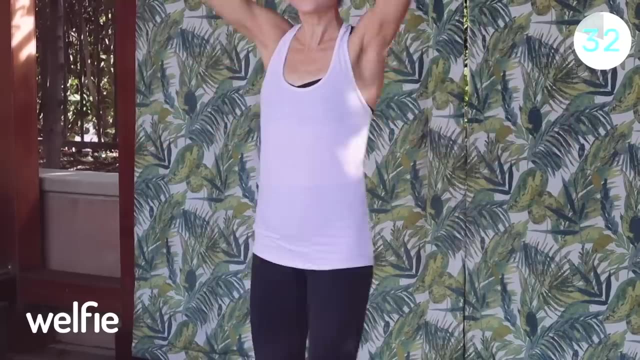 50 seconds in 50 seconds. Knee raise- Now you should feel your heart rate pick up. That's great, You're moving and you're doing excellent. Can you reach those arms up a little bit higher And stand up a little bit taller? Feel free to go slower or just little knee raises. If a big knee 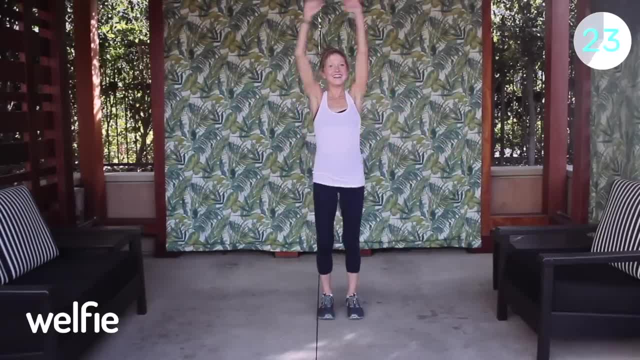 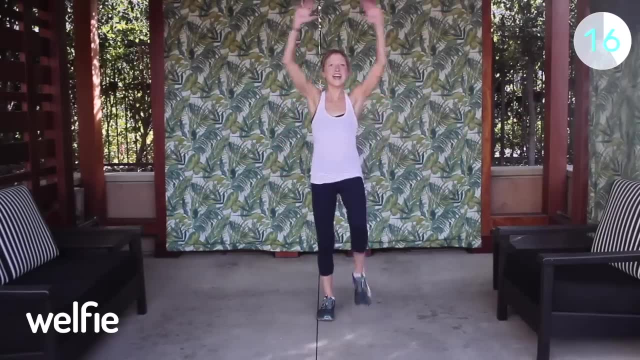 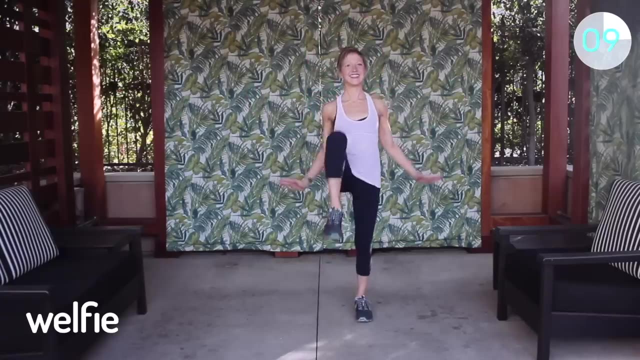 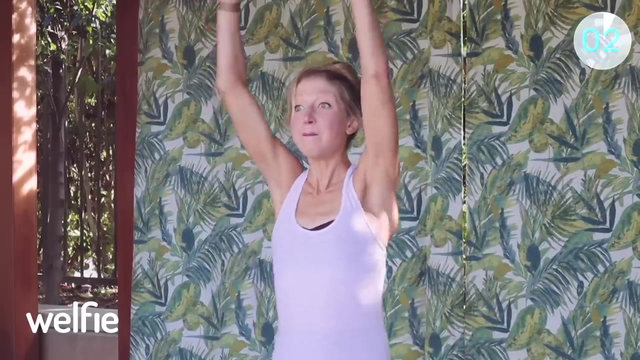 raise is not feeling right for you. Awesome job. How is your posture? Check in. Make sure you're standing up tall. Big arms, Big breath. Good work, I'm so proud of you. Keep it up, Big reach. Whoo, That was awesome. 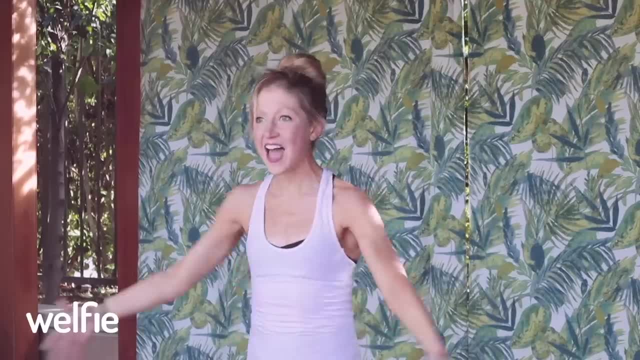 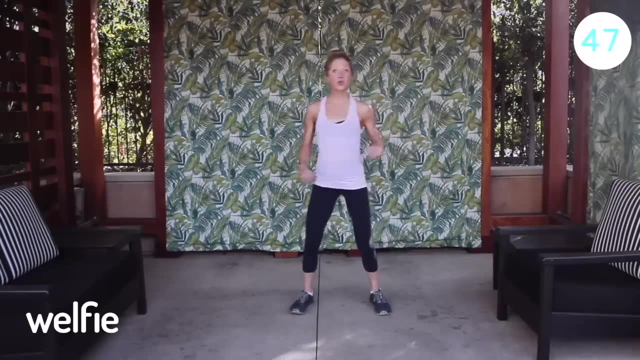 Exercise number three is a boxer. punch side to side Abs, tight arms ready and punch Side to side. Now that you're ready, let's do this one more time. Now I'm twisting through my feet to make this a total body exercise, but if you need something, 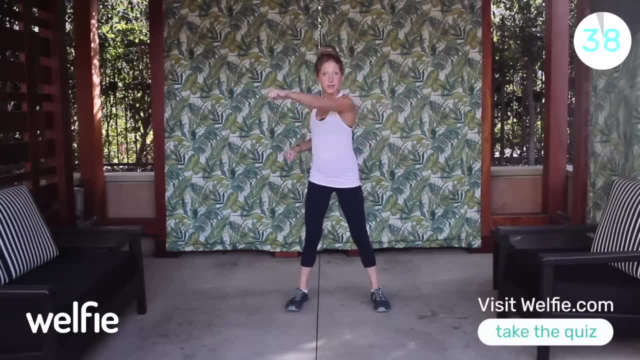 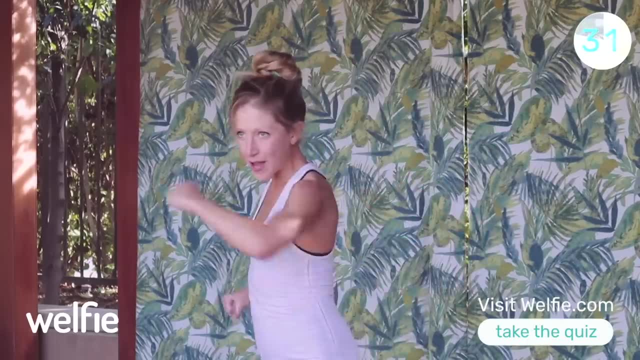 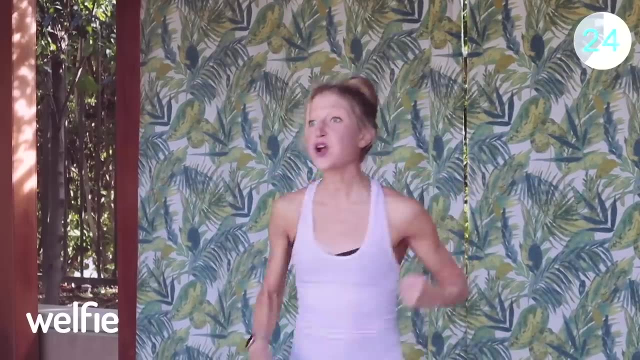 a little bit softer. you can just use your arms, But make sure you contract your core and keep those abdominal muscles tight. Boxer punch: You can punch out any negativity or any things that might be holding you back from your health and fitness. 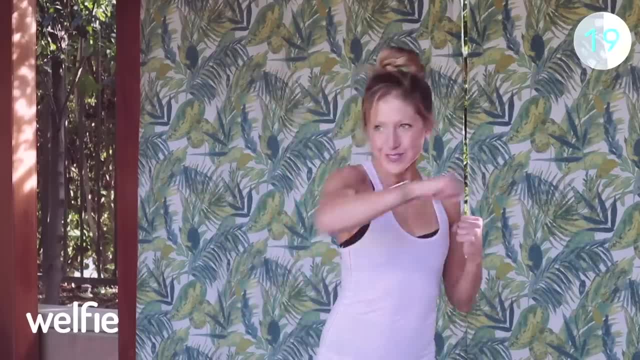 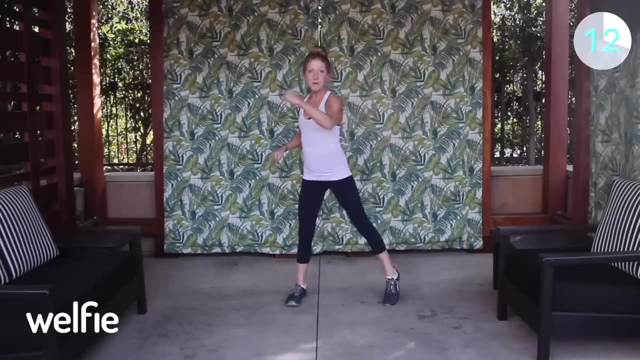 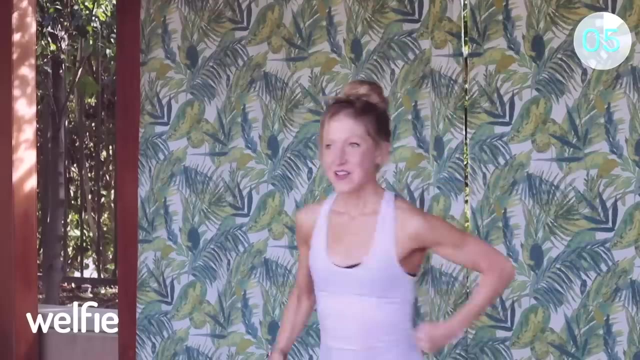 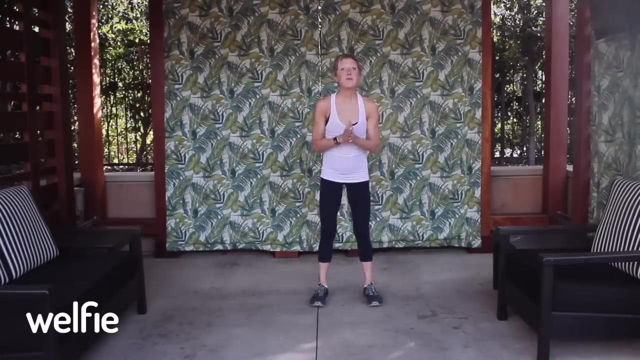 Just get it out of your system. Give me some bigger arms. You're doing amazing. Positive energy fuels the fire, So keep thinking positive and believe in yourself. You can do this. Nice job, Tummy tight Rest. Next up we have lunges. 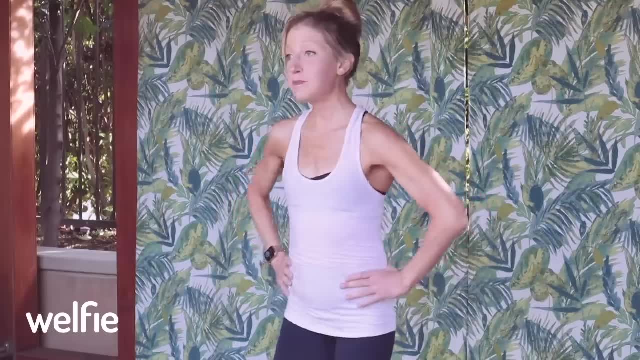 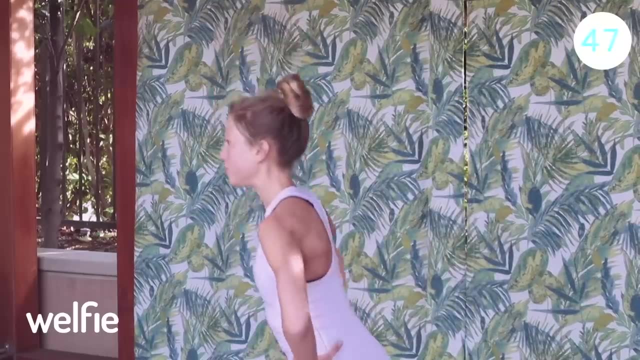 So I'm going to show you a variety of ways to do that. Hands at your hips, Tummy in nice and tight, Stand up tall And you'll lunge back behind you. Step together and switch Now the lunge. you need to make sure you have good form. 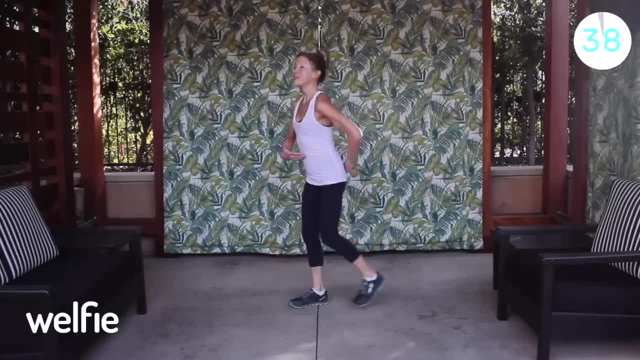 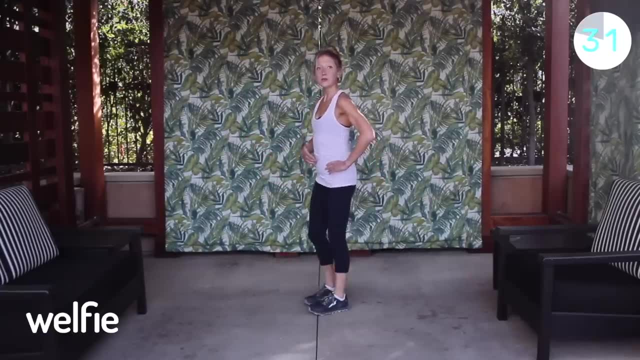 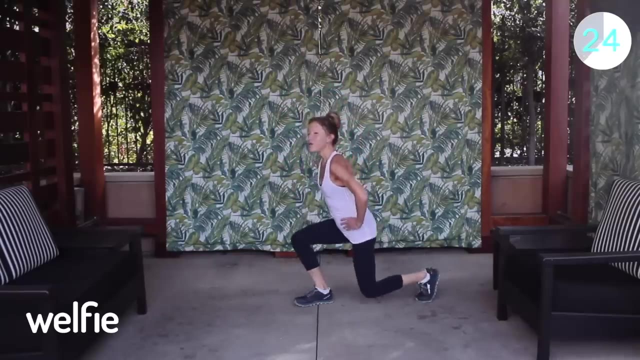 Keep your knee behind your toe Abs in tight Spine straight. If the lunge is a little too much for you today, you can go back to those knee raises that we did earlier. Modify as needed and move mindfully. If you get better at this exercise video, you'll get to the lunge. 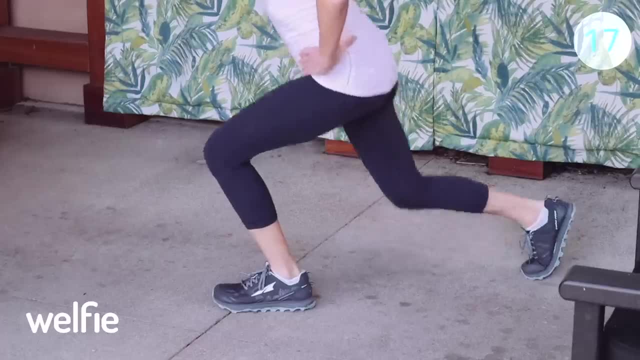 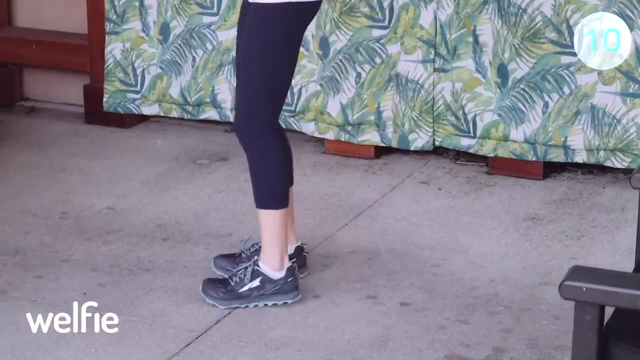 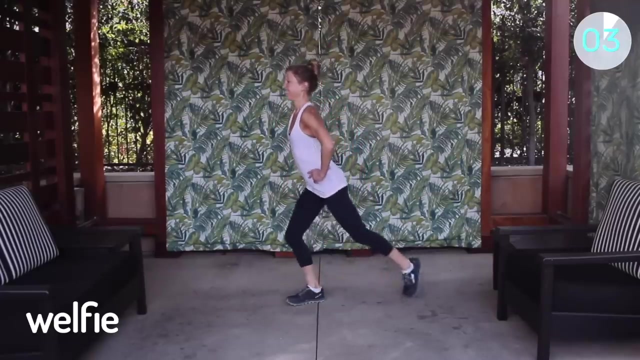 I know you will. It's good to have a challenge to work up to, To get stronger for Beautiful job with this lunge. How is your form? Check in? Your heart rate should be coming up now. Alright, lunges are done. 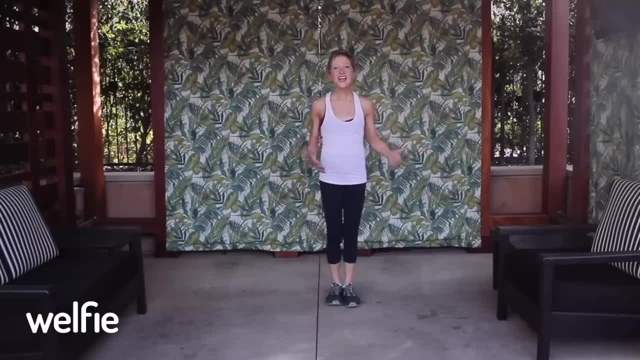 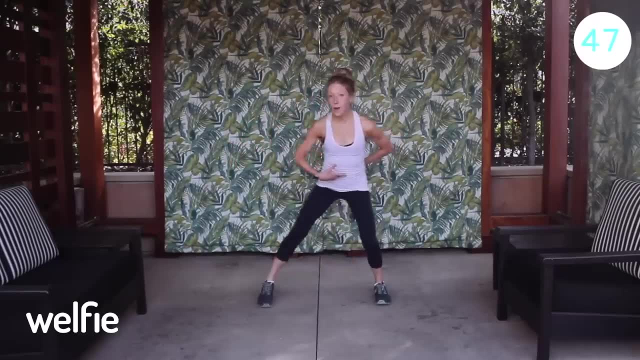 Next we go to a sidestep. This is an aerobic exercise and I know we can do it together. So abs tight, Let's go Step touch. Now I do a mini bend in my knees so that I'm really working my thighs, and because I love 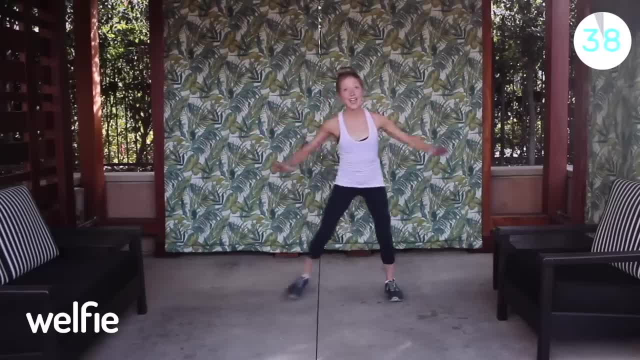 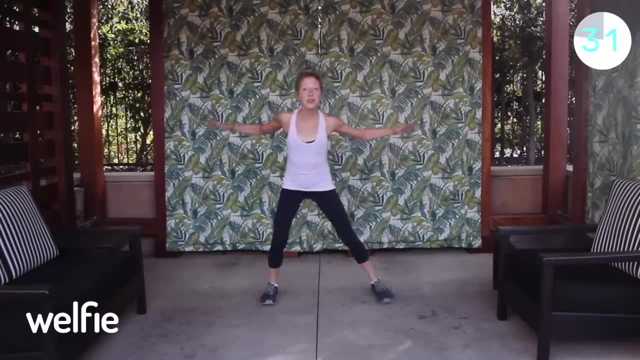 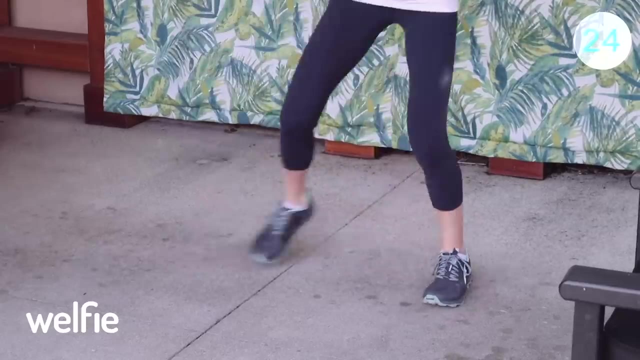 adding arms. I'm just going to reach my arms out to the side and clap my hands in together when I step the feet together. You can do whatever works for you, as long as you're moving and feeling better. as we keep going together, Let's lower the blood sugar, improve your health and make you feel fabulous. 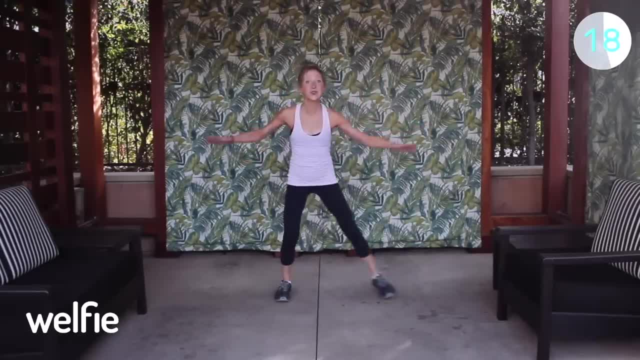 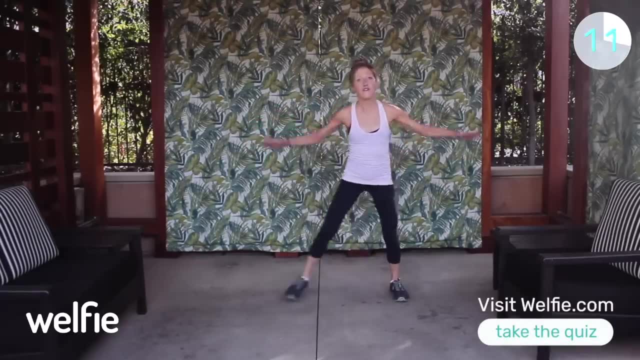 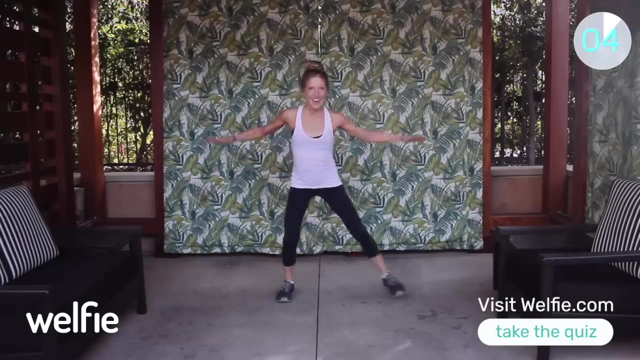 Remember, You don't have to go to extremes to see results. Little bits of movement. This exercise video can go a long way in helping you feel better, quickly and effectively. Good job. Can you get a little lower on this side step? How is your breathing? 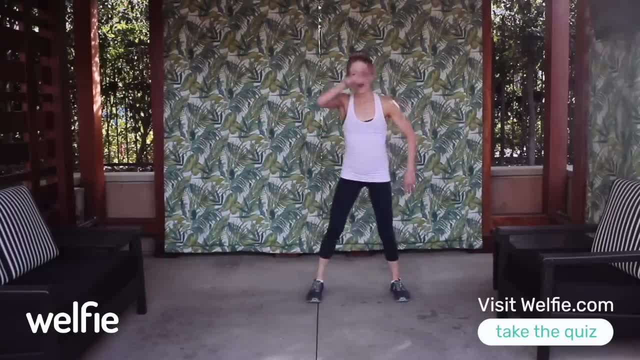 I hope your heart rate's coming up, Whoo Okay. Next up, we're going to work the hips with a hip abduction. Check it out. You stand up, nice and tall, tummy in, nice and tight, and you're just going to reach. 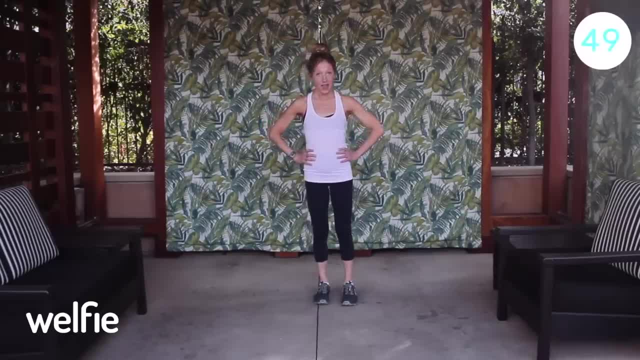 the leg out to the side and switch. Here we go. So when the timer starts, it's your time to shine. Make sure that your toes are pointed straight forward, not up to the ceiling. You want to feel the outsides of your bottom, your hip muscles and your thigh muscles. 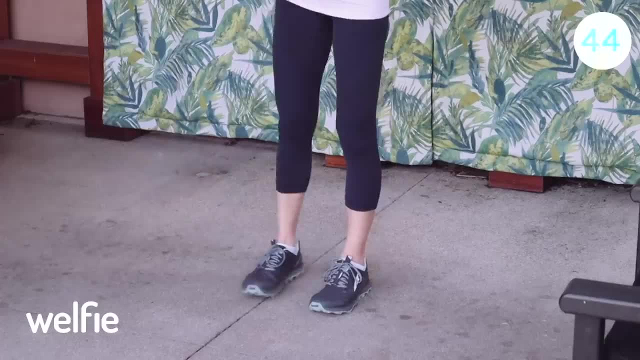 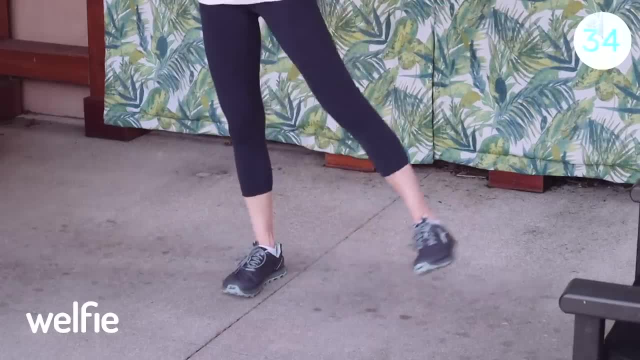 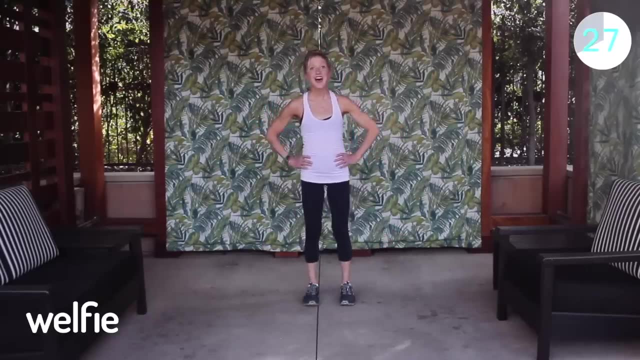 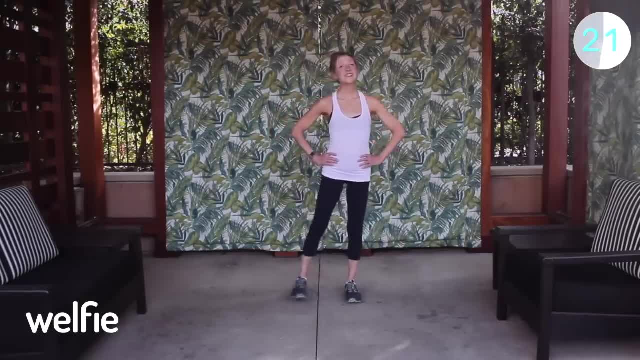 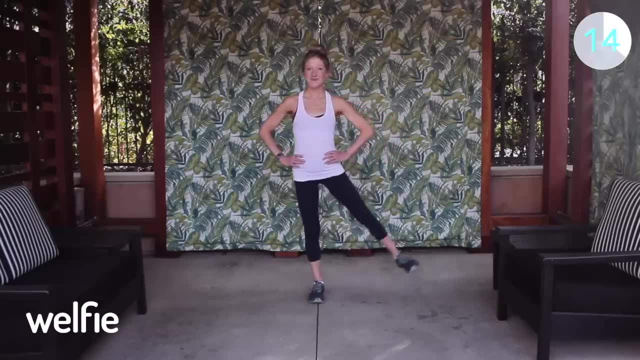 Let's go, Let's go. Good job, You're a pro, A true pro, Way to work through all these exercises. Can you stand up taller? I bet you can. You got it Hang in there. We're almost through this 50 second hip abduction. 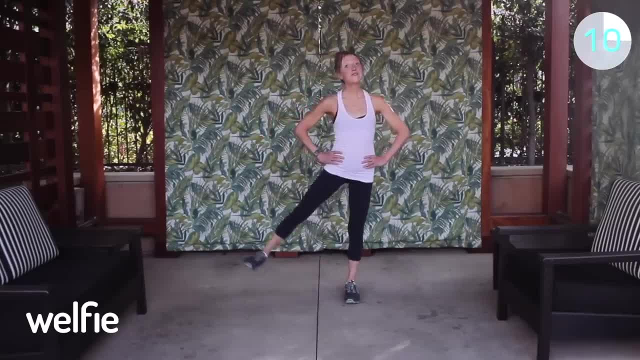 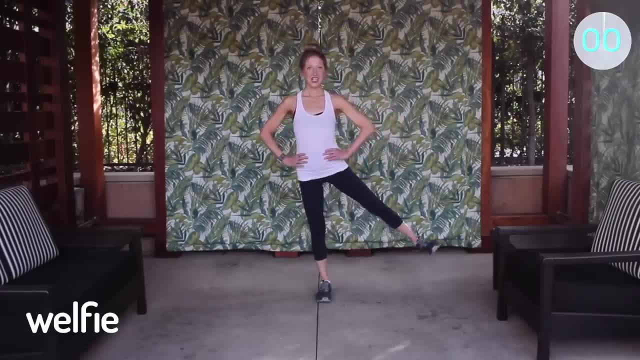 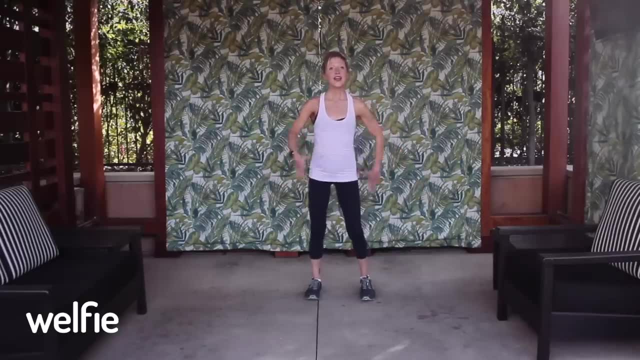 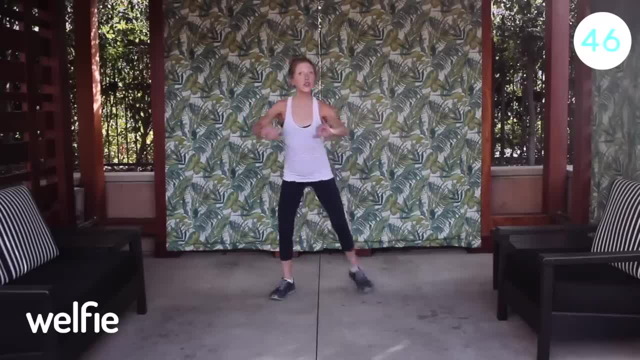 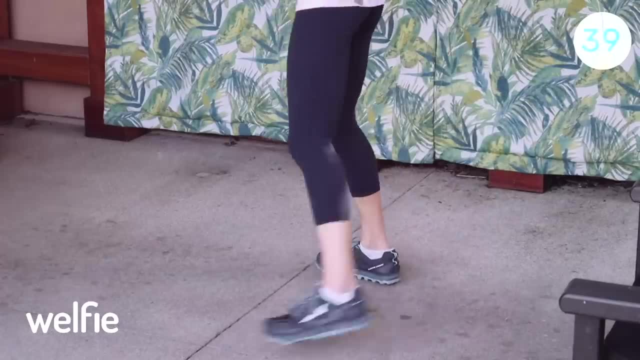 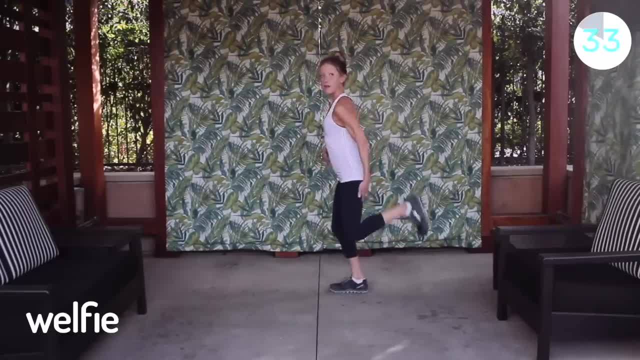 Let's go Ready. It's called leg position. It's a product of the gym. It's a great exercise. It really helps with your blood pressure. so when you're ready, tummy tight, arms forward and you're going to kick your own butt. 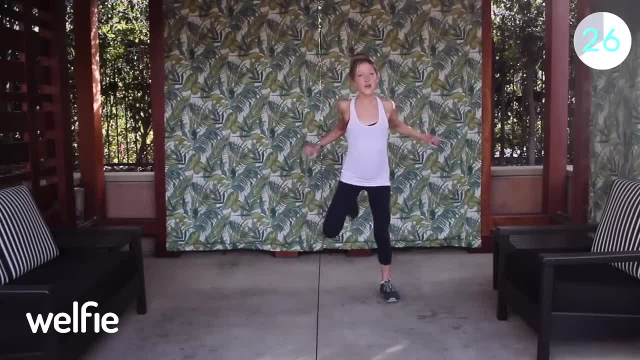 Kick, Kick. I'll show you this from the side. See, I'm curling my hamstring by bringing my heel to my butt. You want to make sure that the knee stays back, back muscles as you bring the elbows into the sides. good, feel free to go. 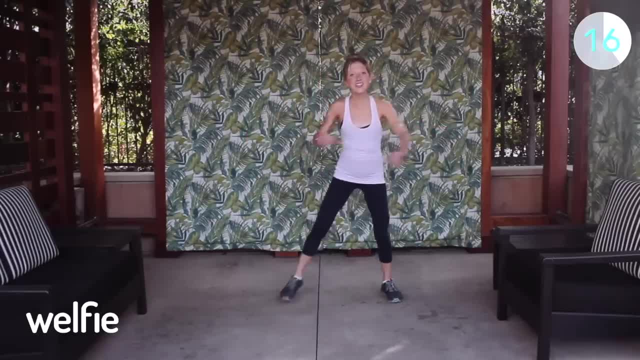 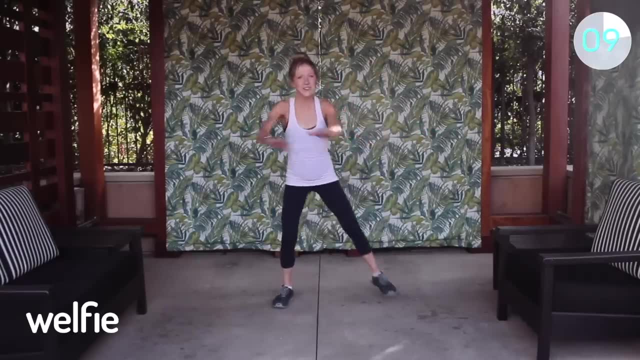 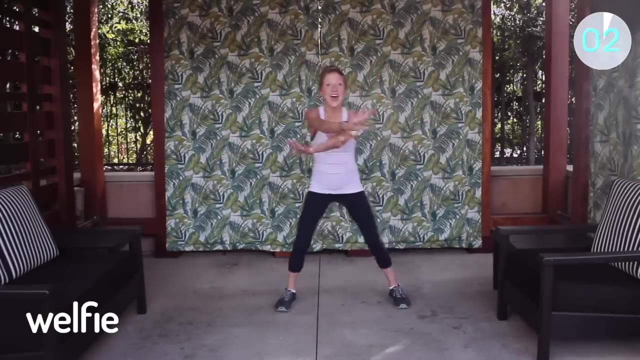 slower or faster, as long as you feel challenged and you're feeling better as we move together. movement is so much better with other people that support you, don't you think I'm here for you and you're doing great good job. give me a bigger hamstring curl, if you can, and a big breath as you keep moving, okay, that. 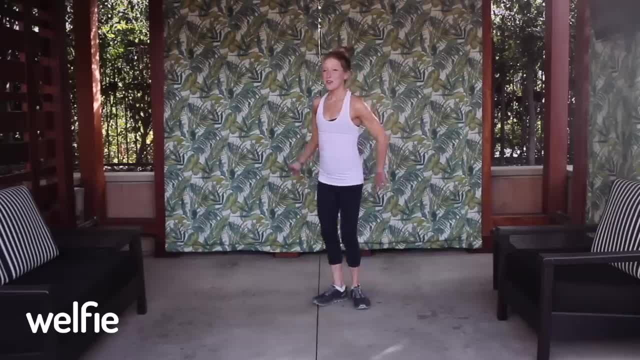 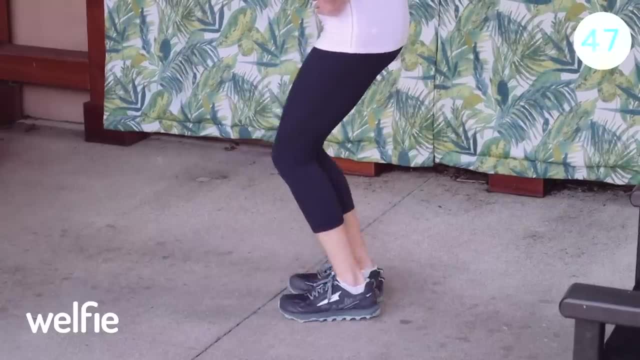 was hard. we've got some heel taps next. this is fun. you're gonna bring your feet together, squat low, tummy in nice and tight and tap so you're staying low in what I call a chair pose. squat, spine is nice and straight and you're doing a. 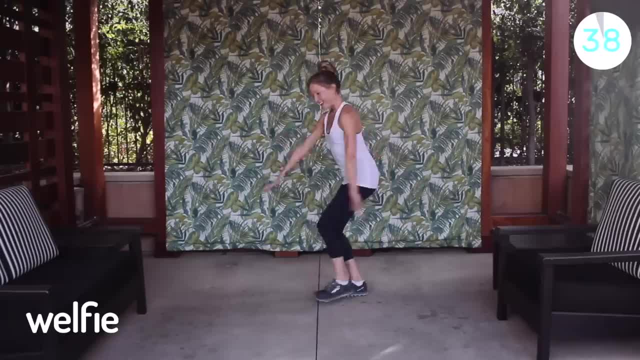 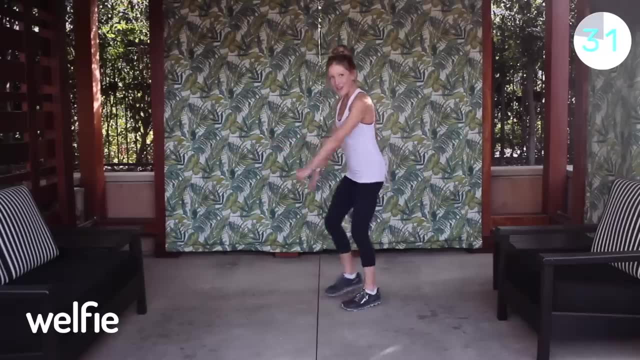 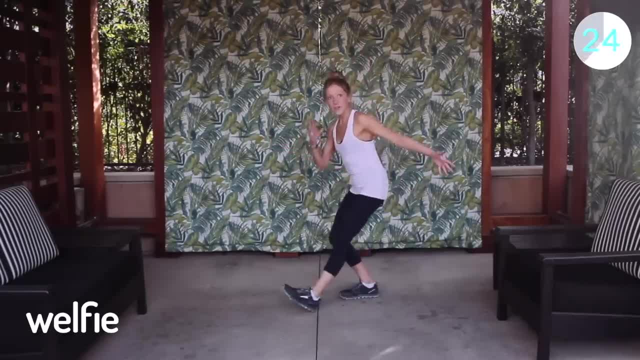 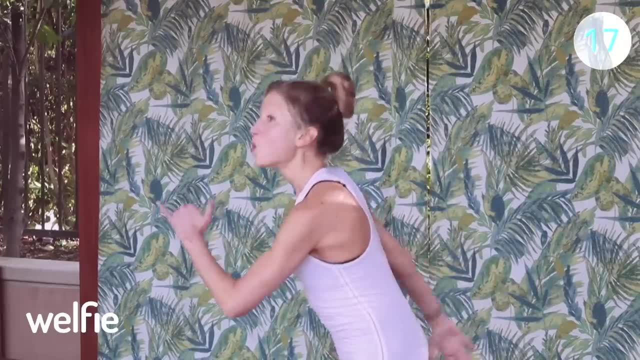 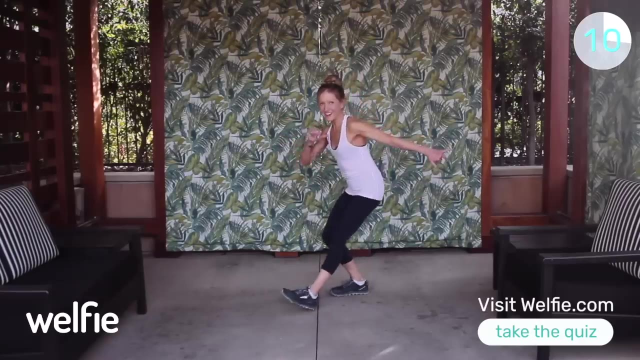 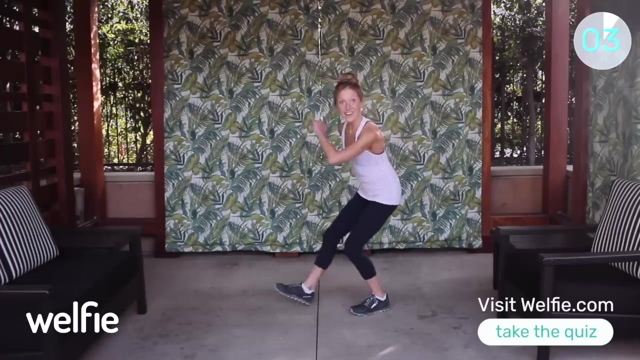 you have to have fun when you're exercising, because if you have fun, you'll stick with it more, and the more you stick with it, the better you feel. exercise will help you feel better. movement is medicine. stay with it. squat a little lower if you can keep breathing. use the arms. nice job, how you feeling? 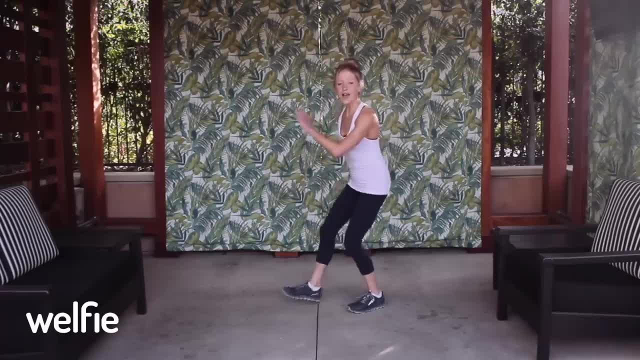 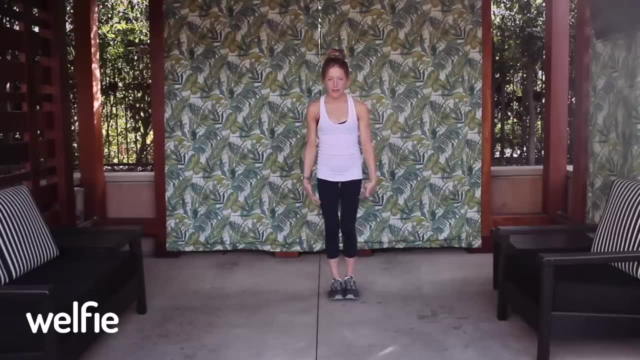 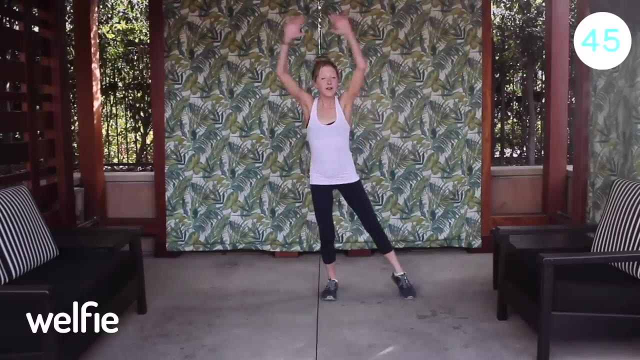 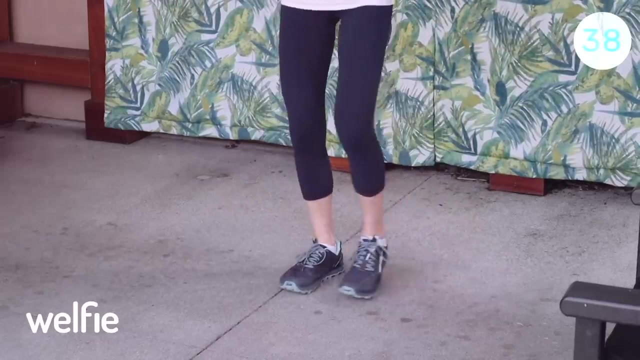 good, stay with that squat and rest. okay, one of my favorite exercises: the modified jumping jack: feet together ready, go arms up, touch the toe out. now we do a modified jack because this is a low impact sequence of exercises to help you lower your blood sugar, not high. 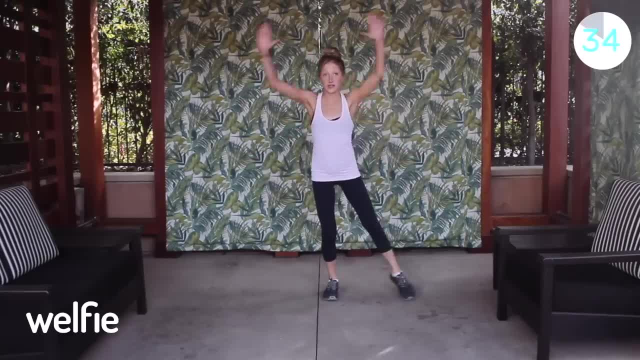 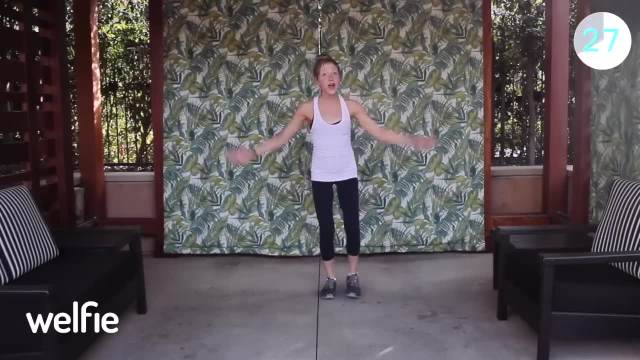 impact, because high impact can be hard on the joints and I don't want you to hurt. after fitness. I want you to feel better. remember your exercise is going to help you feel better. exercises don't have to beat you up. they can actually just make you feel better in your life. 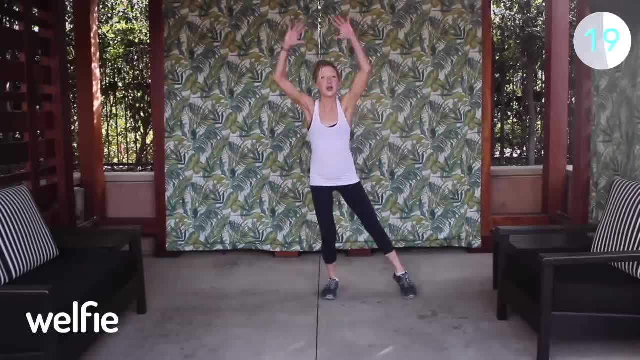 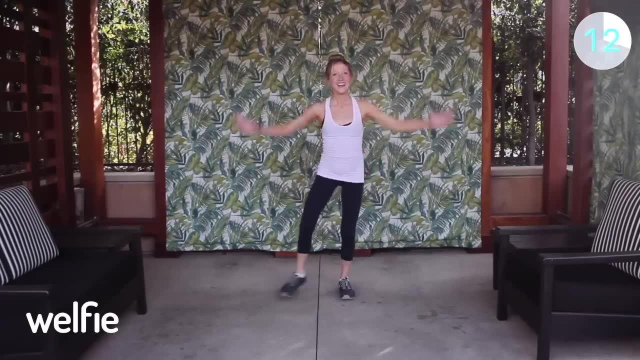 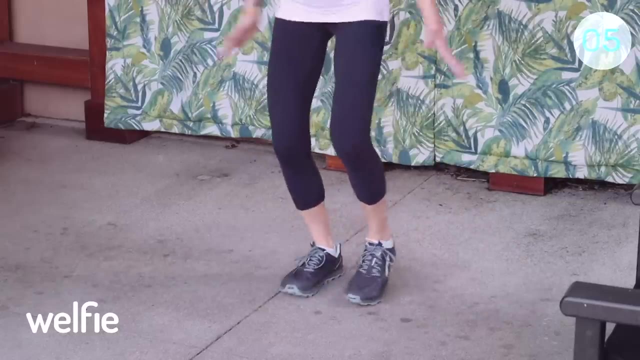 so we're doing all low impact exercises to lower your blood sugar. you can even do this at your apartment and your neighbors won't hear a thing, which is awesome. keep reaching those arms up high and breathe. nice job, my friend. I'm right here with you. can we go bigger on those jacks? you're almost.